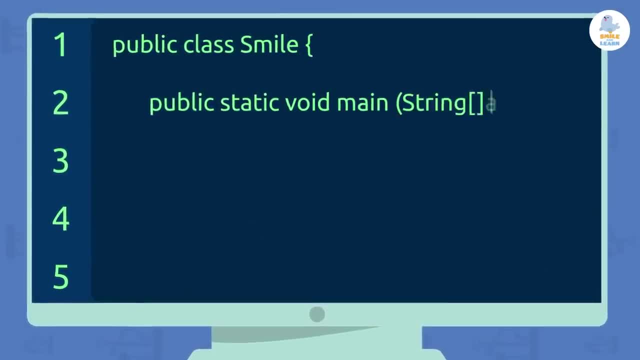 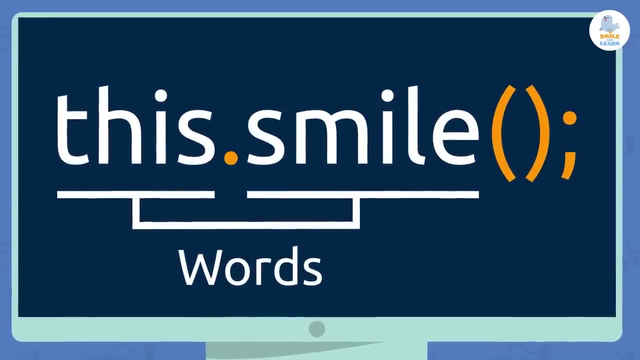 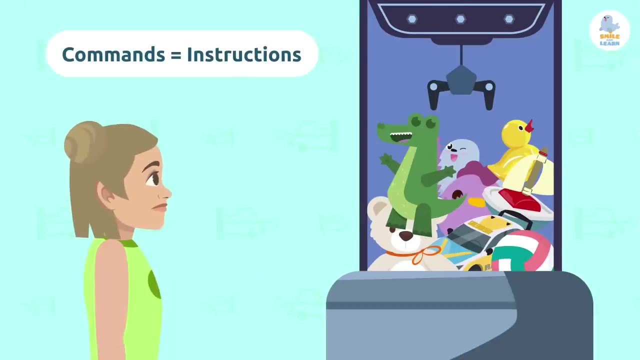 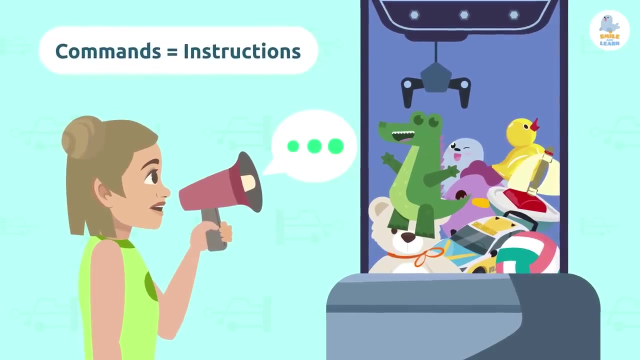 That means there are many different ways to give instructions to machines. With these languages we can write code which combines words and symbols to form commands. Commands are instructions we give machines. They tell machines what actions they should do, and they're different for each language. 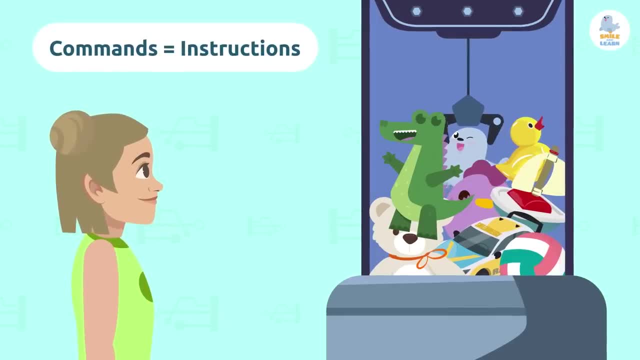 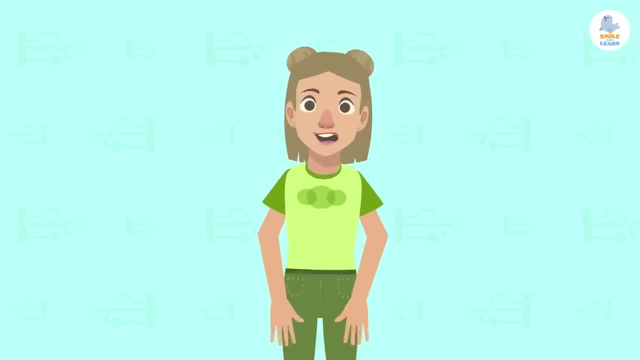 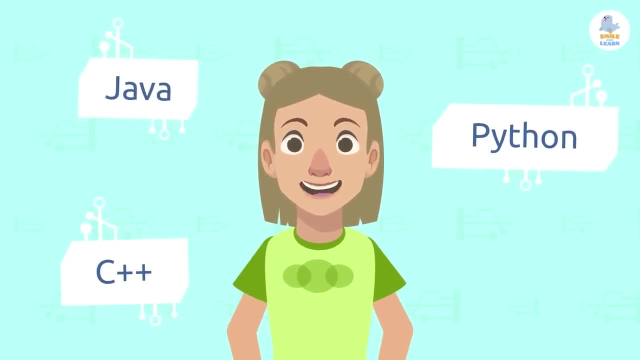 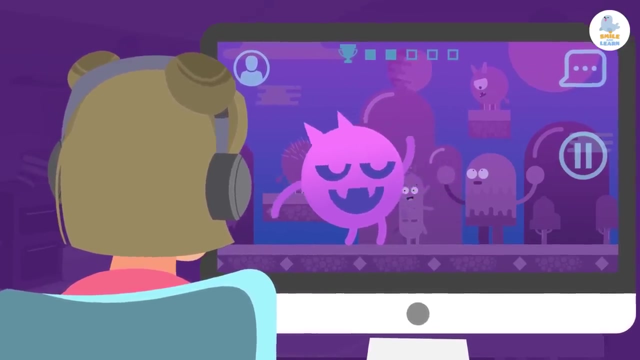 When a computer receives a command, it knows what action it has to do. There are many different programming languages, and some of the most famous are Java, Python or C++, although there are many more. Did you know that these programming languages were used to create some of your favorite video games? 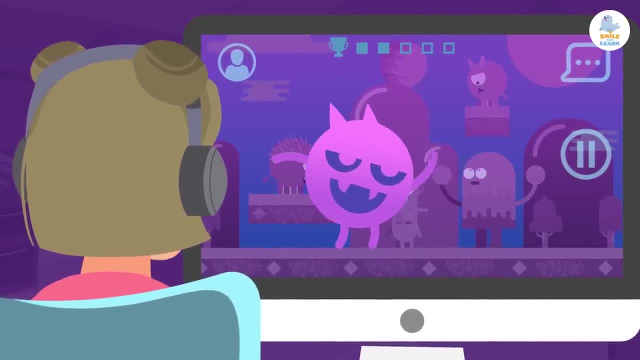 And although there are many different languages, they all use the same programming language. And although there are many different languages, they all use the same programming language. They all use the same programming language. And although there are many different languages, they all use the same programming language. 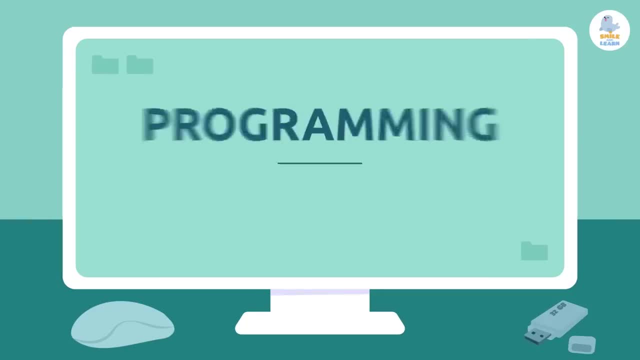 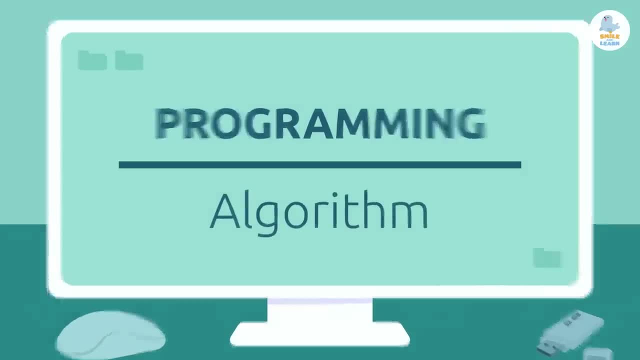 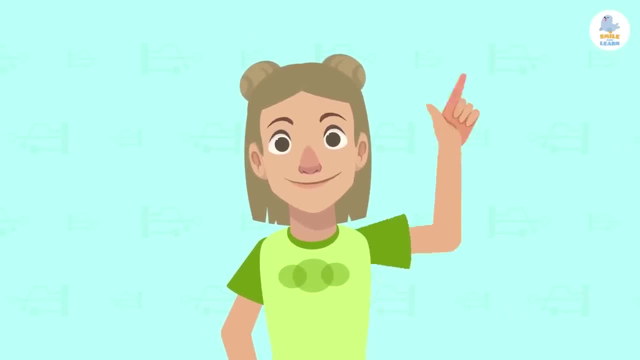 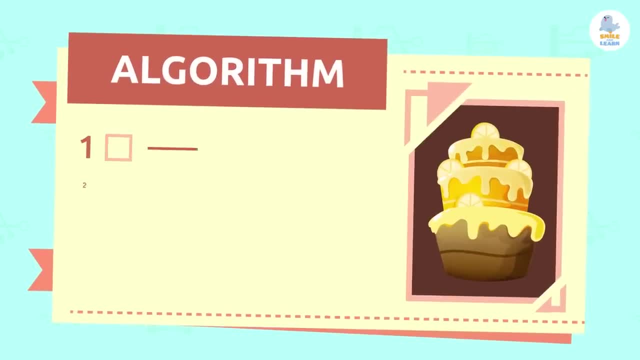 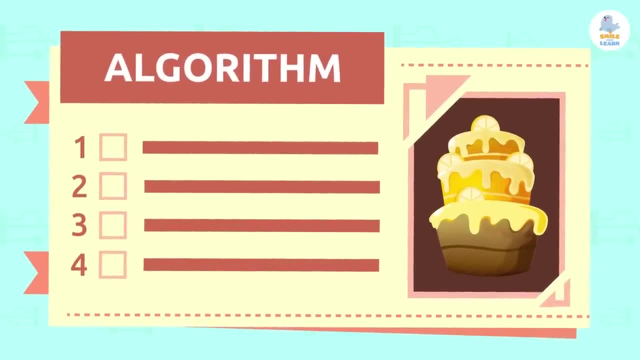 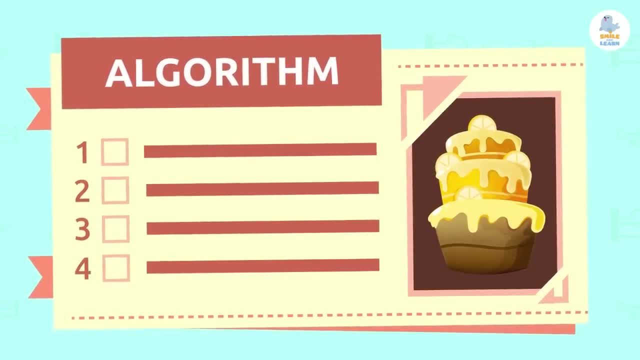 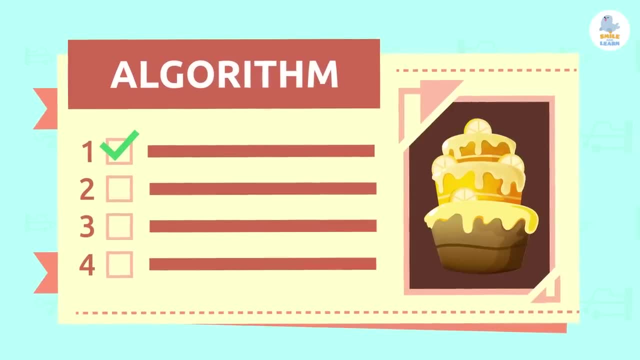 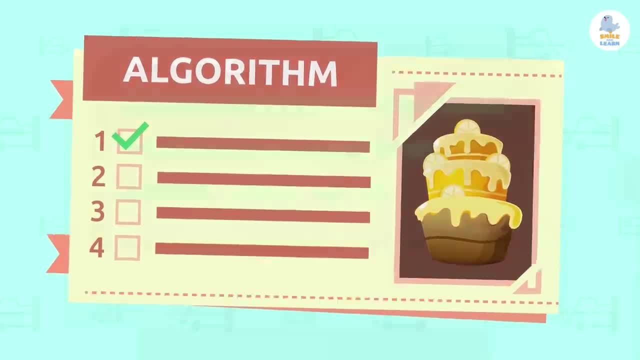 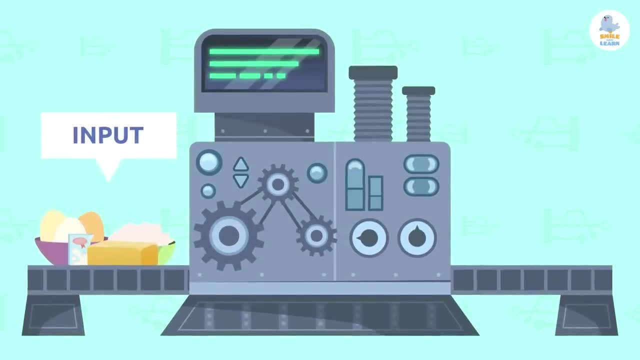 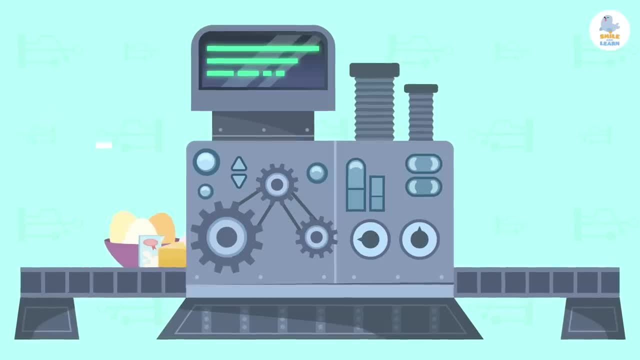 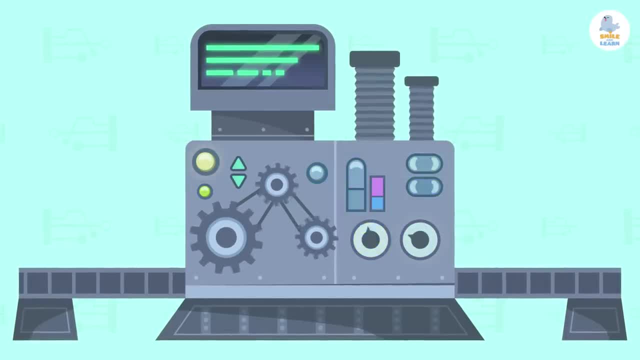 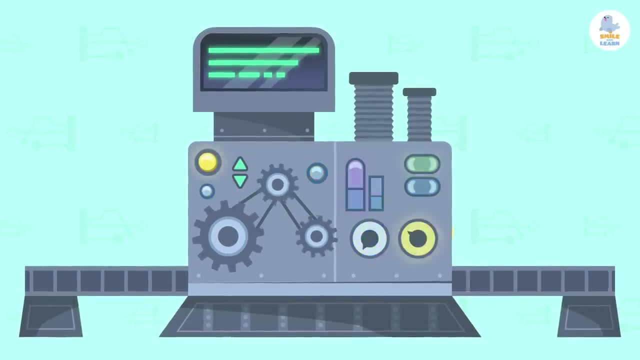 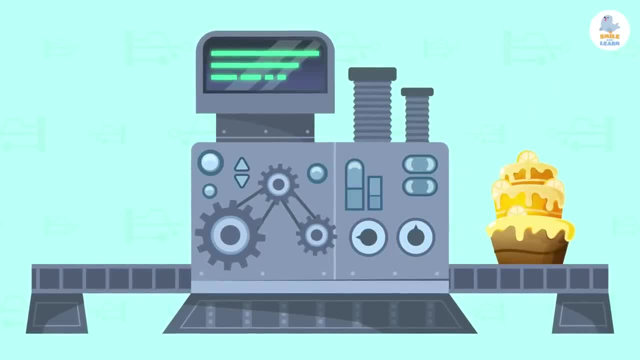 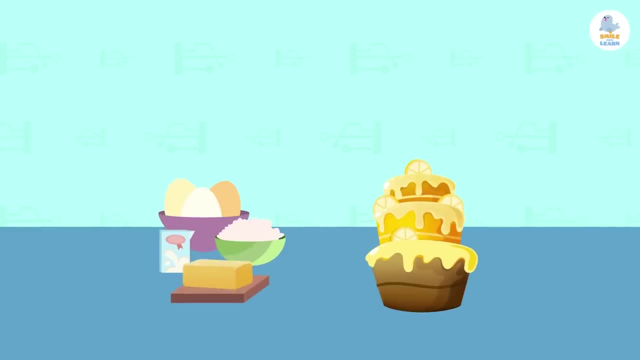 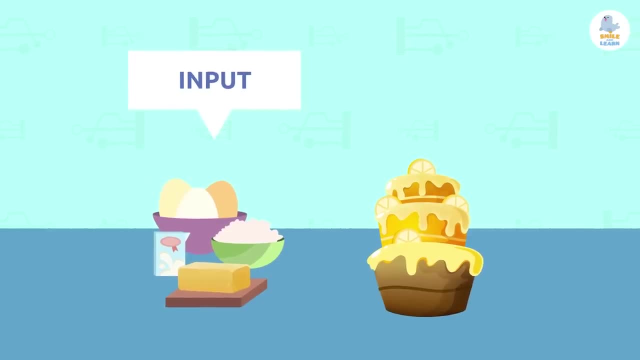 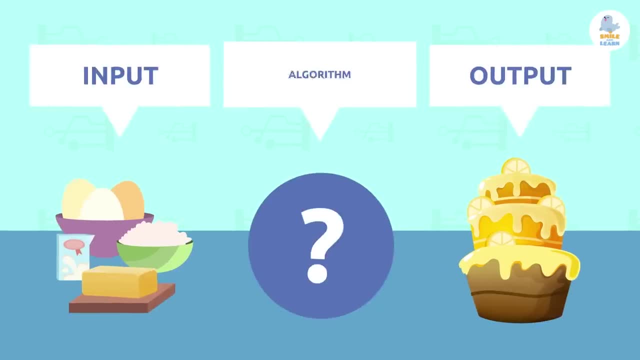 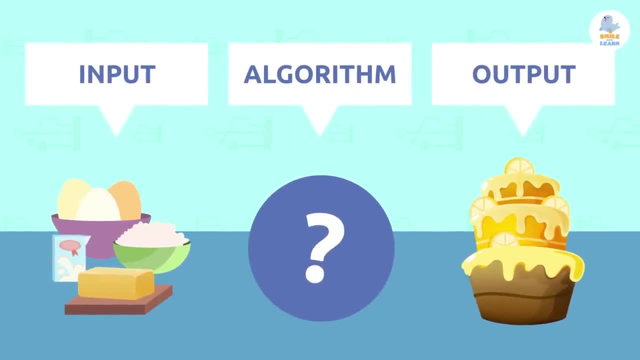 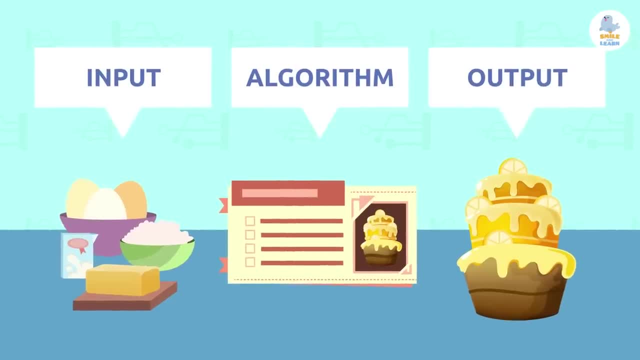 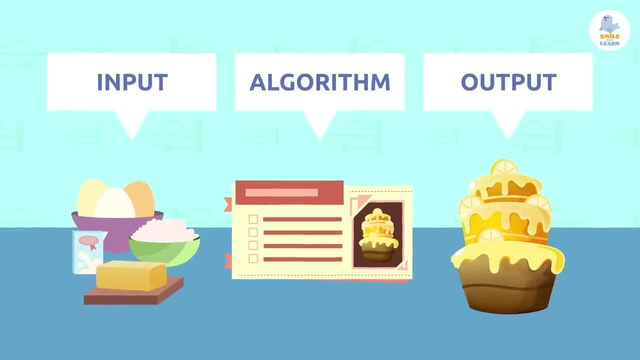 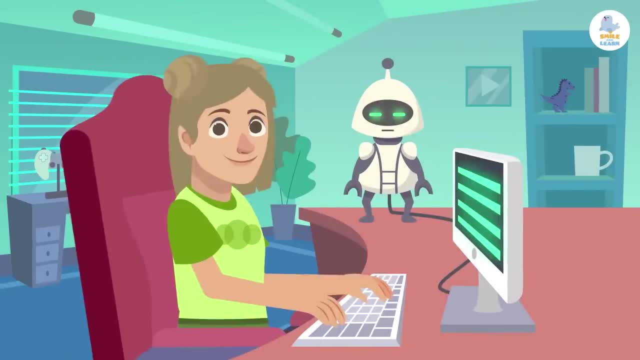 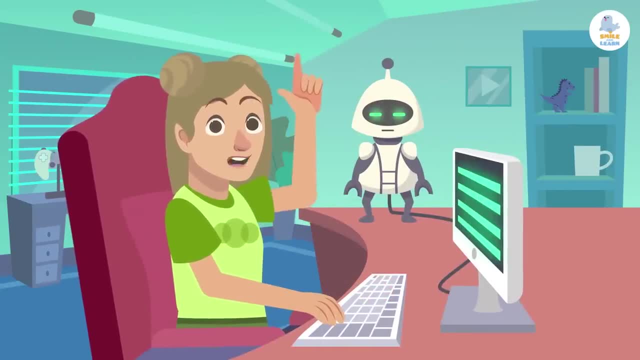 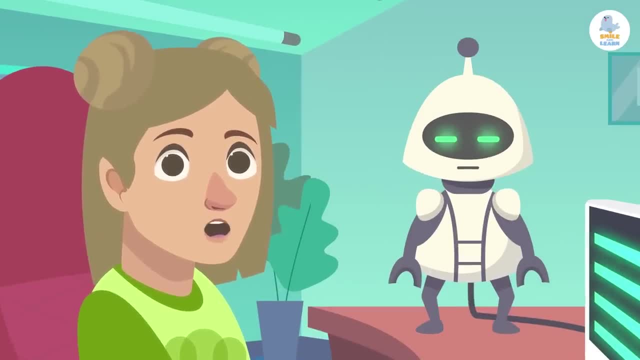 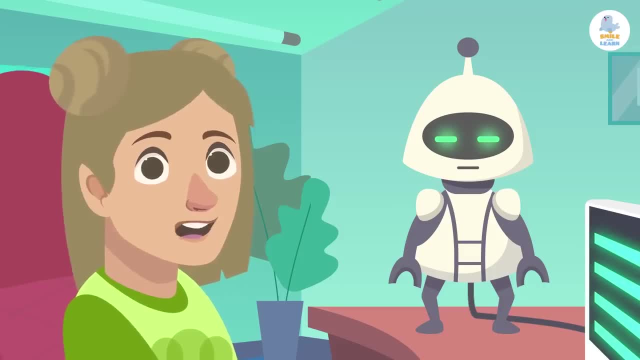 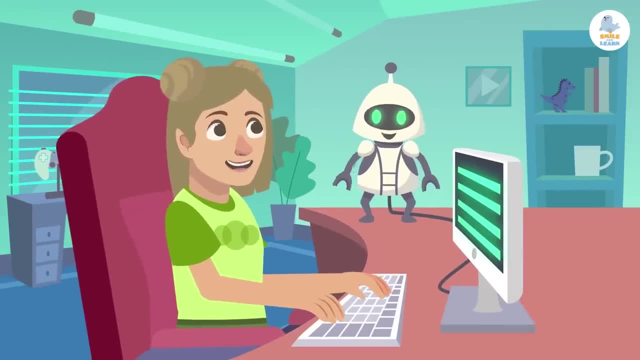 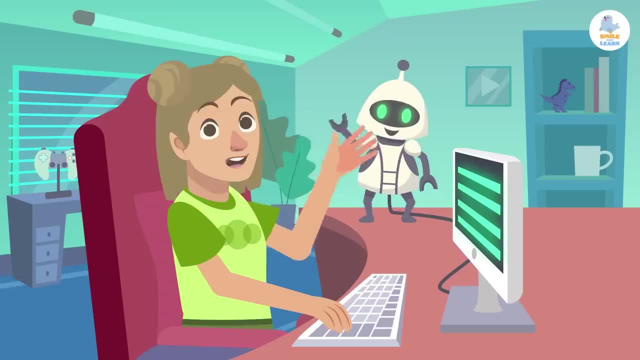